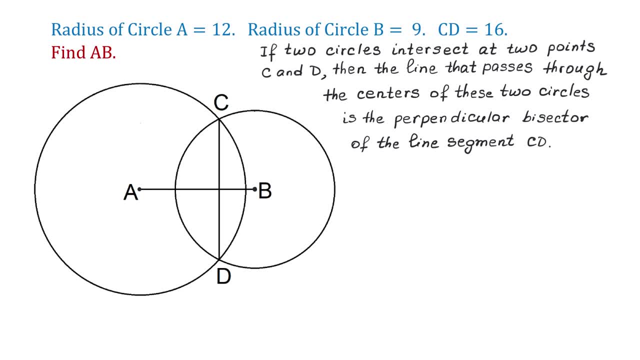 then the following is true: If two circles intersect at two points, C and D- then the line that passes through the centers of these two circles is the perpendicular bisector of the line segment CD. This means that here we will have right angles, and let this point be point E. 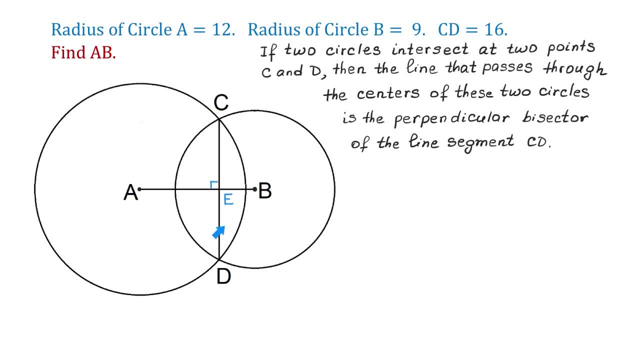 then we can say that CE is equal to DE, and each has the length of 8 units. Now to find the lengths: AB, first we will find AE, then BE, then we will add them together. So then, let's start with AE. For this we will connect A and C, and now we have a right. 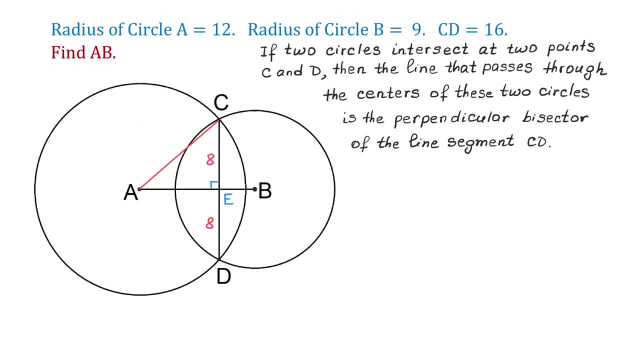 triangle formed AEC. In this triangle AC equals 12, because this is the radius of the circle and CE equals 8.. Then we can use the Pythagorean theorem to find AE. We will write that AE squared plus 8 squared equals 12 squared. then AE squared plus 64 equals 144.. 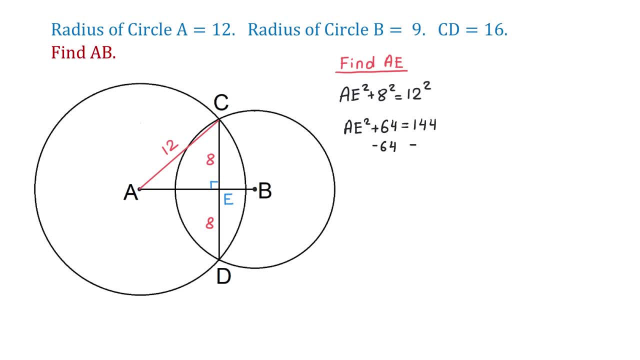 Then we will subtract 64 from both sides. then AE squared plus 64 equals 144.. AE squared equals 80.. Now to find AE, we will take the square root of 80.. Then, to simplify this radical, we will write 80 as a product of 16 and 5.. 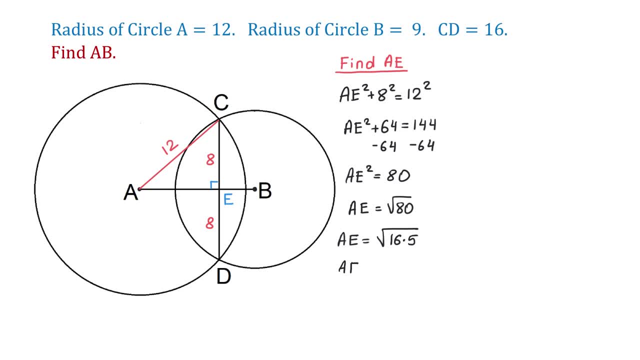 Then square root of 16 is 4, and AE will be equal to 4 square root of 5.. So we just found AE and now let's find BE. For this we will connect B and C and we will have another right triangle formed. 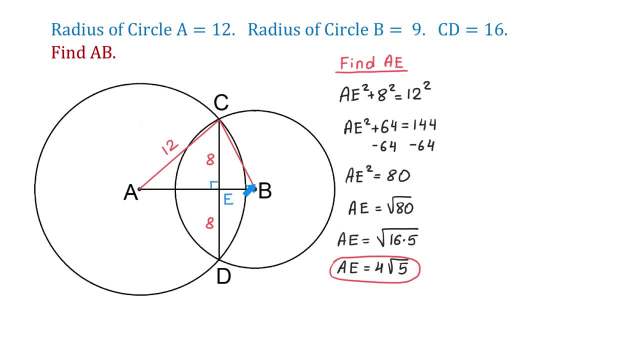 BEC. In this triangle, BC equals 9, because this is the radius, and CE equals 8.. Then again we can use the Pythagorean theorem to find BE. So we will write that BE squared plus 8 squared equals 8..